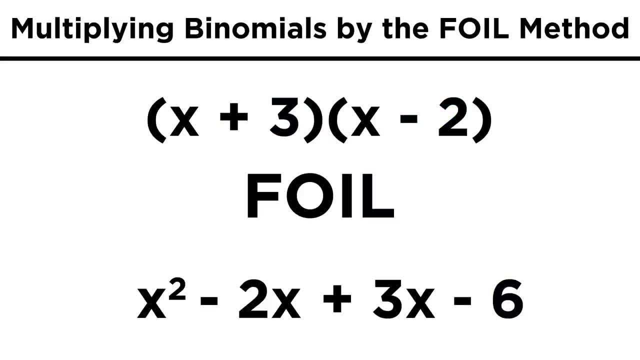 That gives us x squared minus two, x plus three, x minus six, and we can combine like terms to get x squared plus x minus six. Again, the reason this works is because it's as though we are distributing each term of one binomial across the other binomial, and the FOIL method just ensures that we do it. 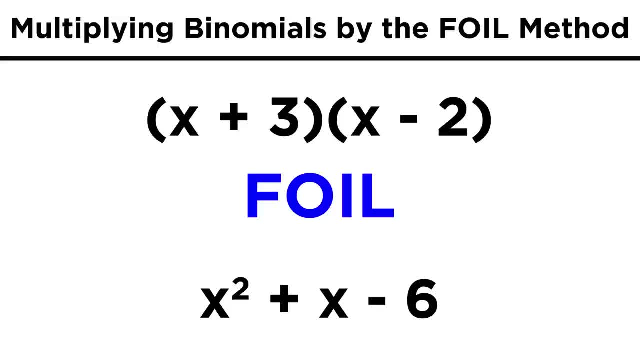 the same way every time, so that we don't make a mistake. The most common error when FOILing is certainly listing the wrong sign for a particular term. Don't get confused by the plus or minus in between the terms of the binomial just. 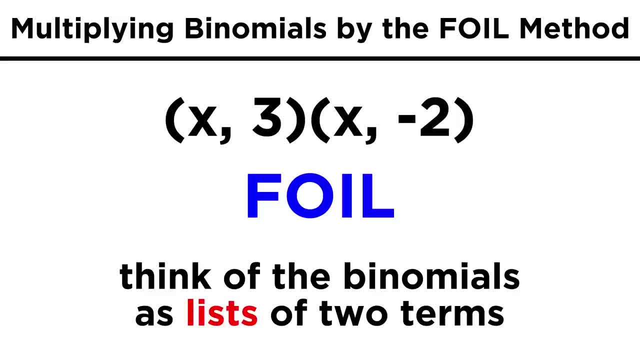 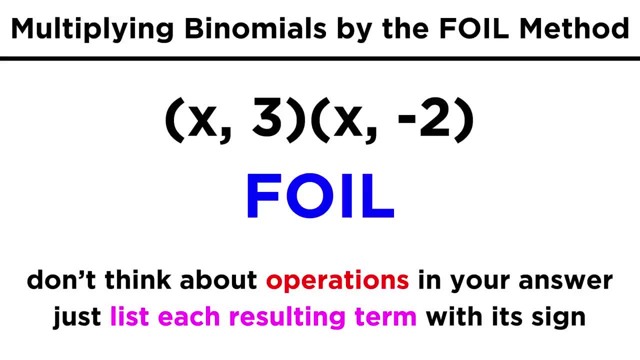 think of the binomial as a list of two terms, each with a particular sign. When multiplying terms, don't think about whether the terms in the resulting list will be added or subtracted. Just list them, The result with its sign, whether positive or negative, and the operations will take. 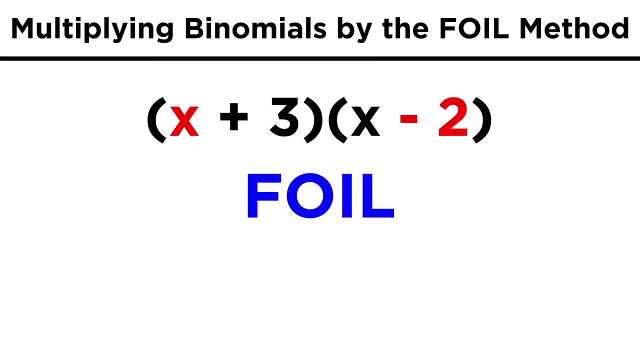 care of themselves. For example, when we did the x times two, just assume that this minus sign means negative two, and when we get negative two x, we just place it in the list For three times x. we got positive three x, so just list positive three x with a plus. 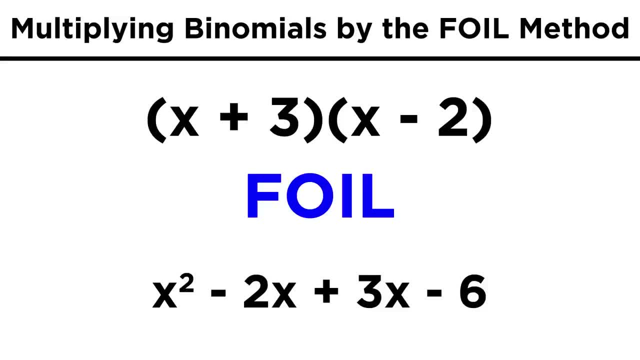 symbol At the end. all the operations are there for us to follow, Clear as day. So if you use this method, it will be hard to make a mistake. Let's try a trickier: one x squared plus four times negative. two x minus one. 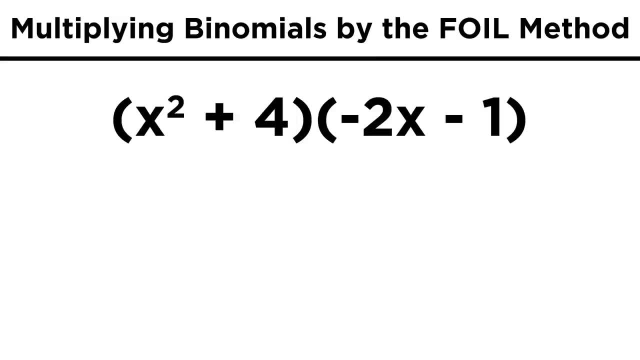 These binomials look different than the previous example, but we still just FOIL as usual For the first term. we get x squared times negative two x, which is negative, two x cubed For the outer. since there's a negative one, we get negative x squared. 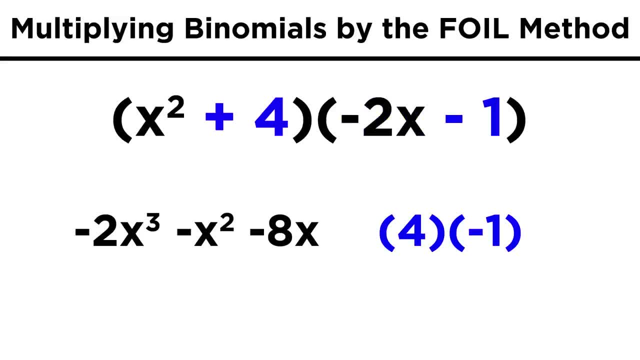 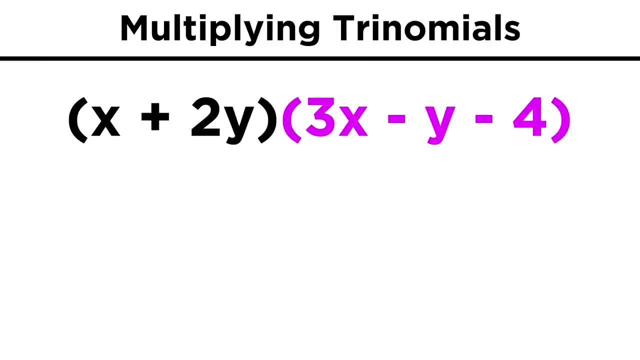 Then inner, There's a negative eight x And lastly, four times negative one is negative four. There are no like terms to combine, so that's the end of it. Now that we can multiply binomials, what happens when we multiply a binomial by a trinomial?